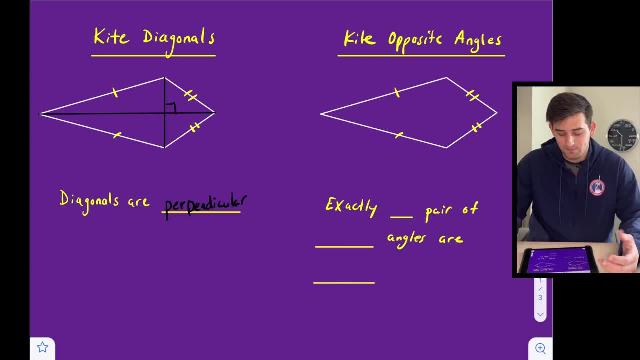 For a quadrilateral to be a kite or a property that a kite has, is that it only has exactly one pair of opposite angles that are congruent. So one pair of opposite angles are congruent, Okay, So, for example, we could say that this angle and this angle are congruent, And if those two angles are congruent, 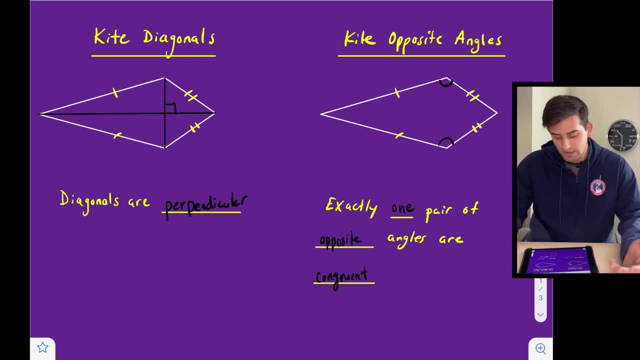 then the other two angles cannot be congruent. Okay, So that could work the other way. We could say that these two angles are congruent, but if that's the case, then these two angles are not congruent. Okay, It just kind of depends. 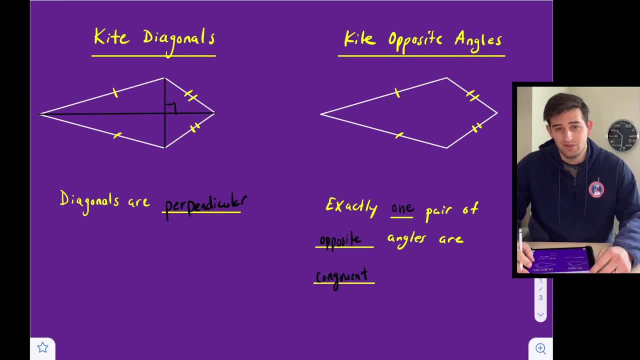 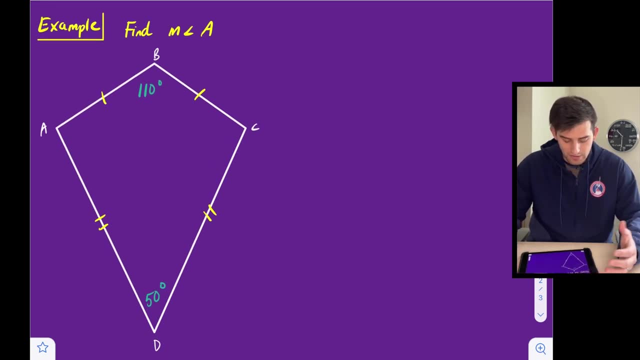 On what the diagram looks like. what information has been given to us? Okay, So with that information, let's do one example here, talking about the angles. So we see we have kite ABCD and we want to find the measure of angle A. Okay, So what we're given is angle B and angle D. 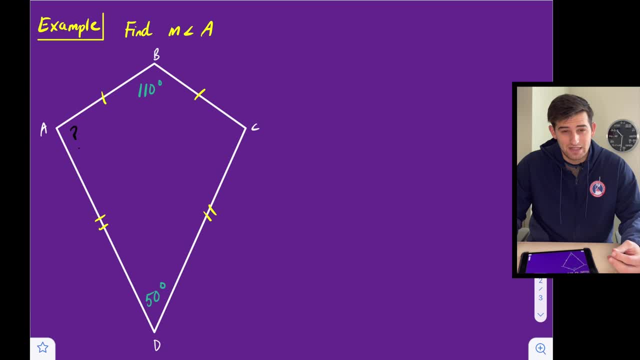 And we know that one pair of opposite angles has to be congruent. Well, angle B is 110 and angle D is 50. So obviously those two angles are not congruent, which means angle A must be congruent to angle C. So now we can use what we know about the angle addition for a 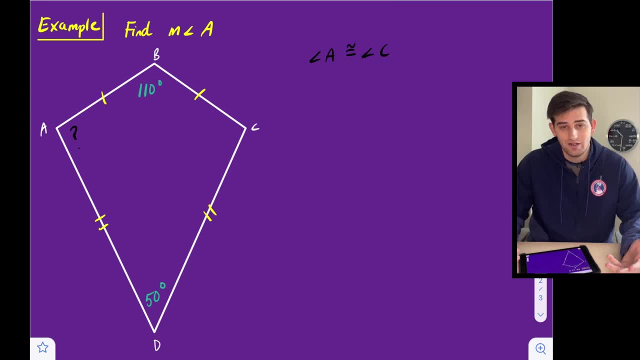 quadrilateral right. We have four sides. So the angles, the interior angles, add up to 360 degrees. So I know I can have 110 degrees plus 50 degrees plus, and let's just call angle A and angle C X, right, They're X degrees. Okay, I'm using a variable X there. We don't know what the angle. 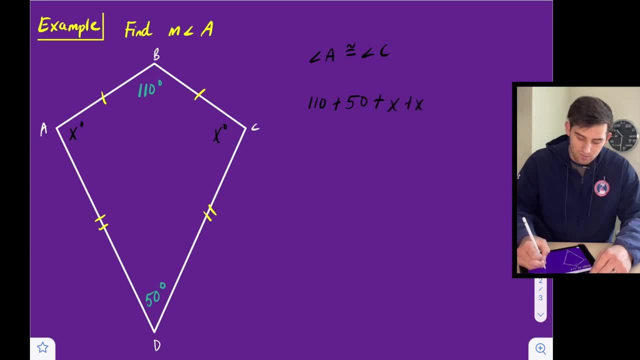 measure is, but we do know that those two angles are the same. So we could say: plus X plus X equals 360 degrees. So now we can combine like terms. So right here we've got 160 plus 2X equals 360, subtract 160 from both sides and we get 2X equals 200. 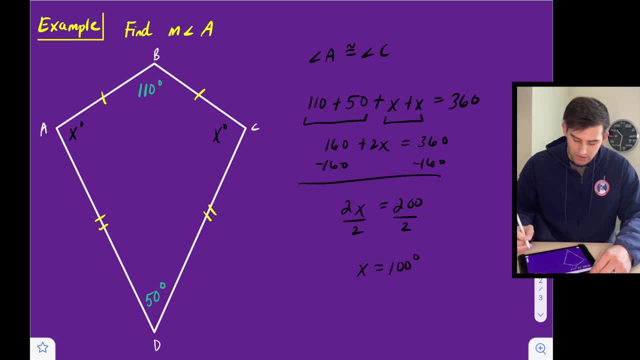 And now we can divide by two to get X equals 100 degrees. Okay, So now we know that the measure of angle A is equal to 100 degrees. Okay, So A is 100.. B would also be 100. And we could check that by adding all four of those together and it. 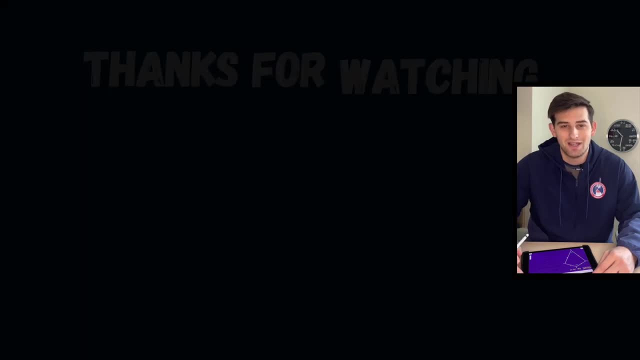 should equal 300.. Okay, So thanks for watching. Those are some properties of kites.